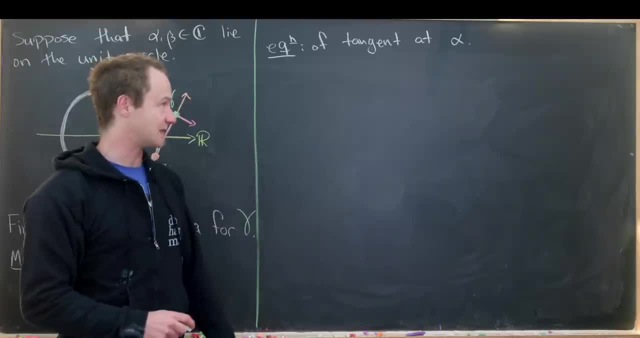 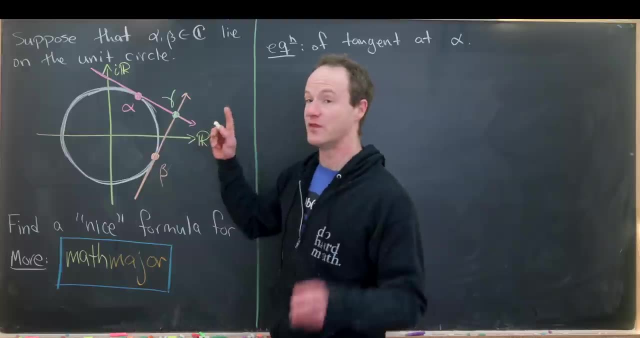 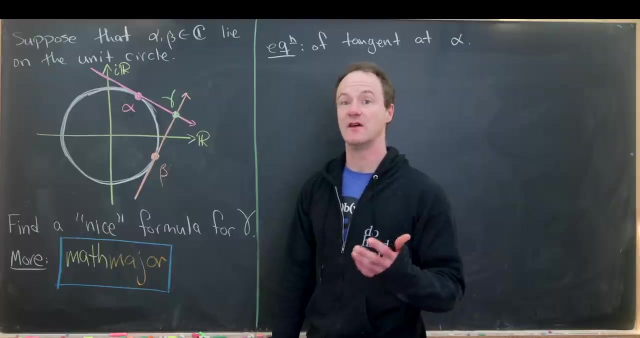 is on the unit circle, And it goes without saying that I'm saying the tangent to the unit circle. Okay, so how can we do this? Well, we need to find out the direction of this tangent line. So the notion of the direction of the tangent line would be like a vector pointing in the direction of the. 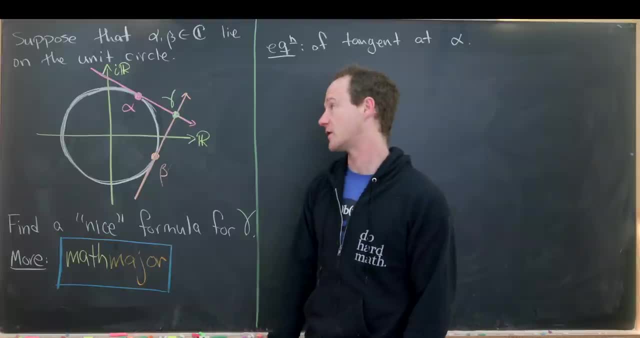 tangent line if we were talking about R2 or vector calculus, Or it would be like the slope if we were talking about single variable calculus. But direction is just given by a complex number if we're talking about a single complex variable. Okay, so how can we find that? Well, we'll 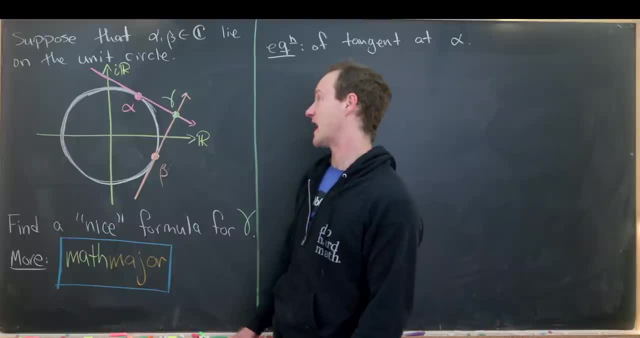 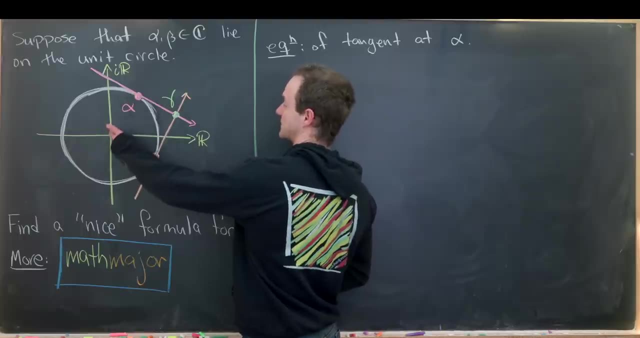 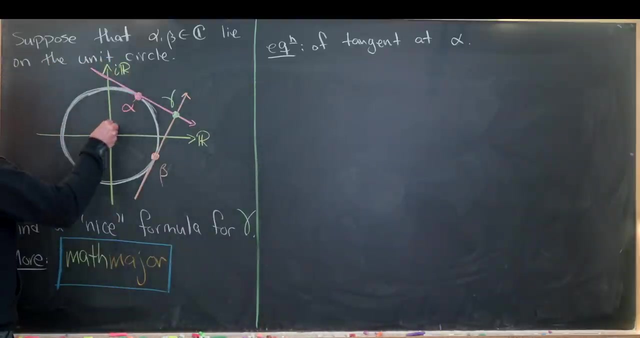 use this kind of really well-known geometric fact that the tangent line to a circle is always perpendicular to the radius of a circle or to a radius of a circle. So if we take a radius from the origin to this point alpha, so that would just be a line segment from. 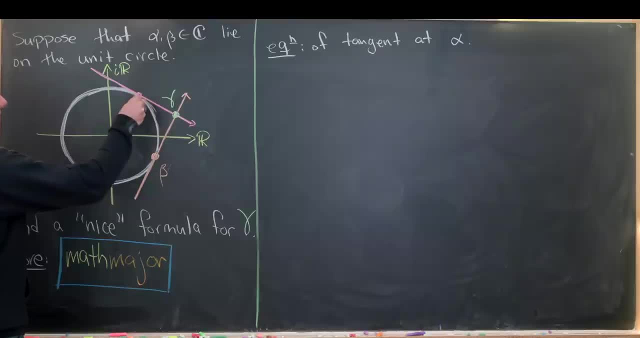 0 to alpha. we know that is going to be a perpendicular line segment to this tangent line, And so this line extending out of this line segment is in the direction of alpha. So we need to find something perpendicular to alpha. But we can do that by rotating alpha by 90 degrees. 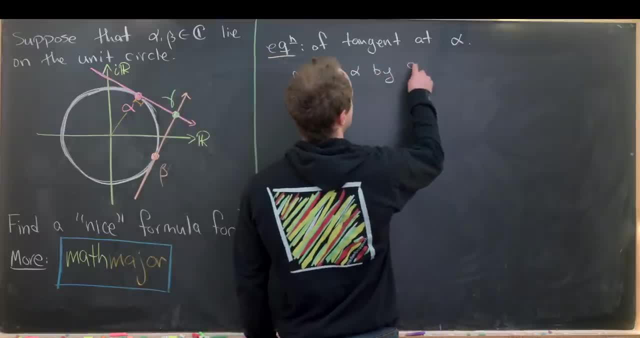 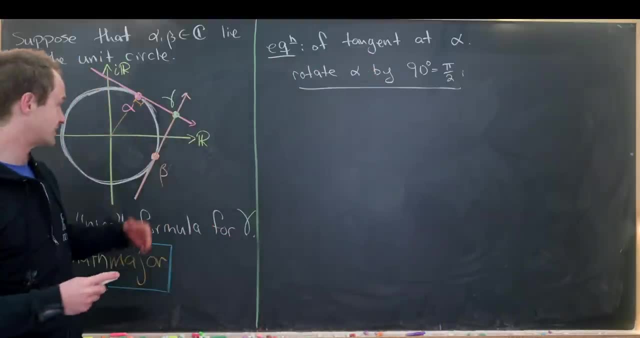 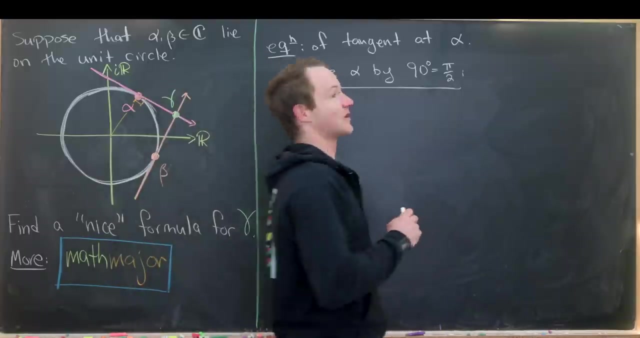 So if we rotate alpha by 90 degrees or pi over 2 radians, then we're good to go and we have a direction for this tangent line. But it's well known in complex variables that multiplication by the number i provides a rotation by 90 degrees. 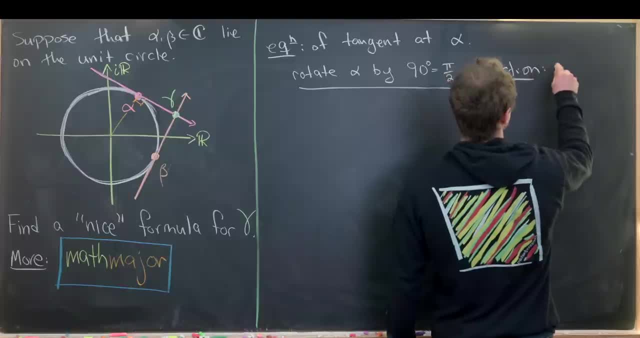 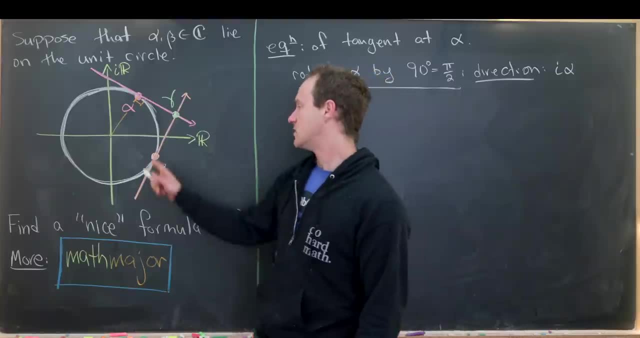 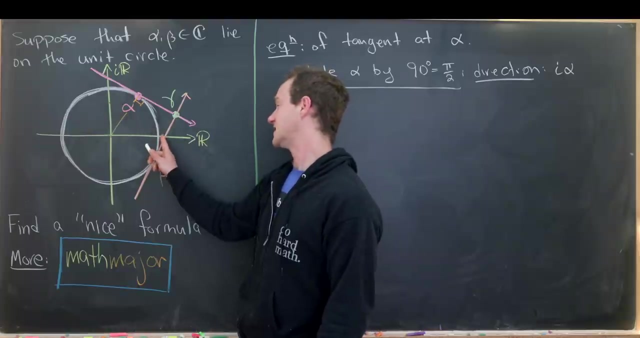 So that tells us we have a direction for our tangent line, given by i times alpha. Okay, well, we can talk through that a little bit. Notice, if we multiply any real number by i, we end with a pure imaginary number, And that rotates this from the real axis up to the imaginary axis. 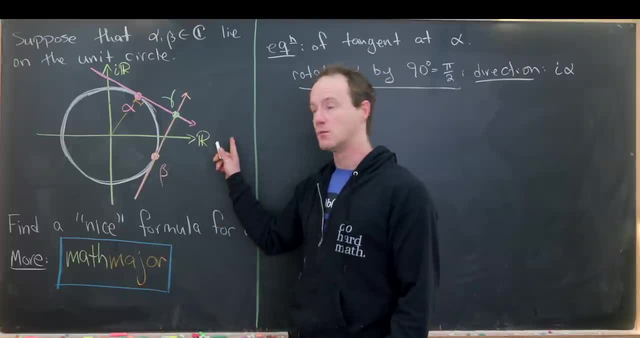 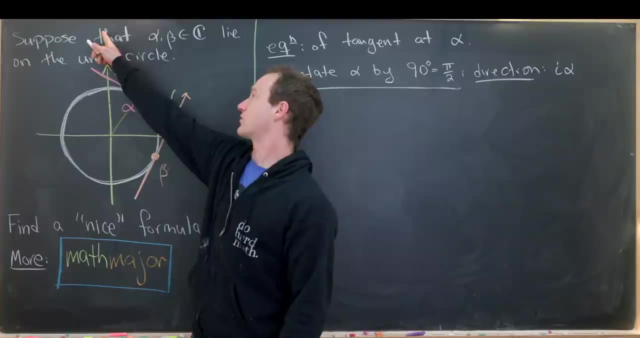 For instance, the number 3, which would be out here, multiplied by i would be 3i, which is up there. That's a 90 degree rotation. Then, furthermore, the number 3i multiplied by i would give us 3i squared or negative. 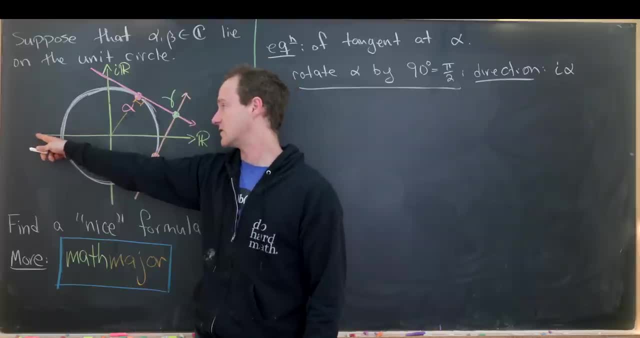 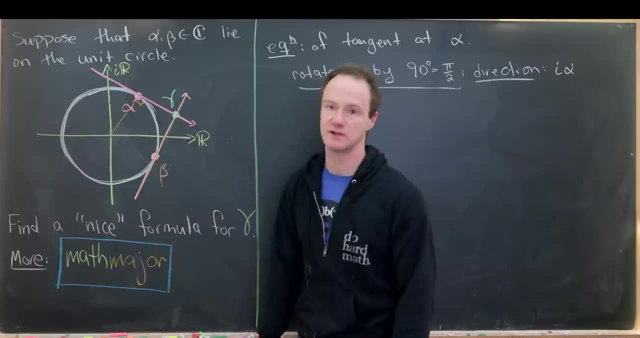 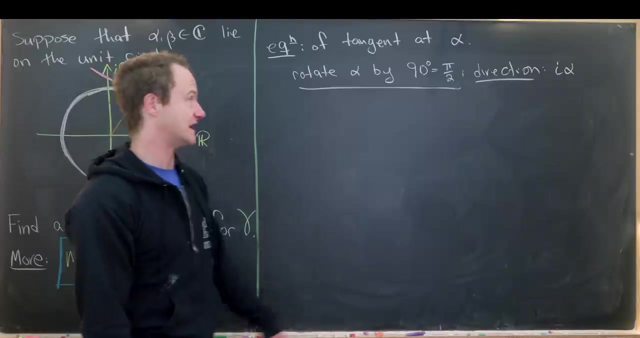 3, which would be back here. That's another rotation by 90 degrees. So you can see that that most definitely works on the axes, but it in fact works anywhere in this complex plane. Okay, so we've got a direction for our tangent line and we also have a point on the tangent. 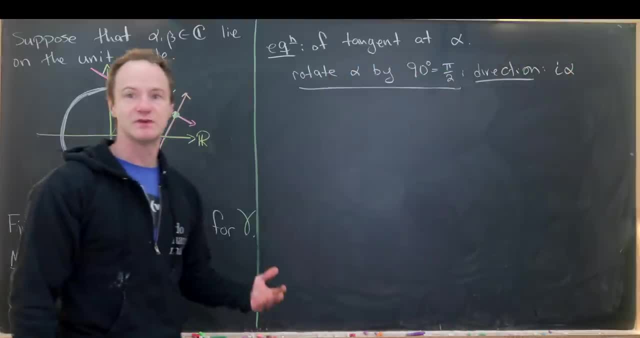 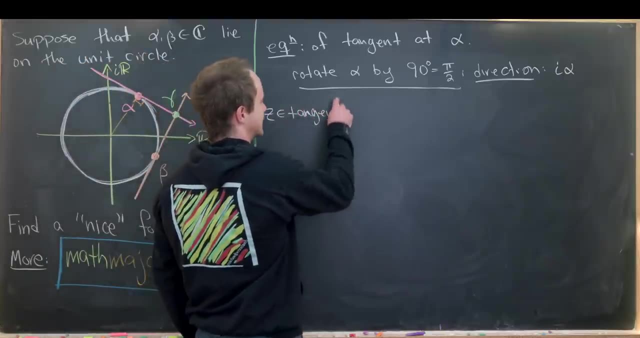 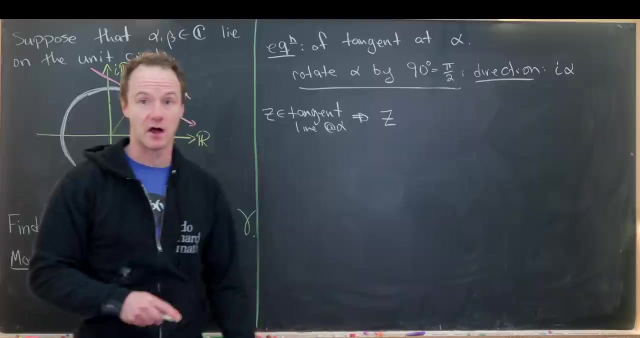 line. So this is a point, this is a direction. So that means we can parametrize this tangent line. So if z is on this tangent line, so I'll just say z on the tangent line at alpha. that means that z must satisfy the following equation: 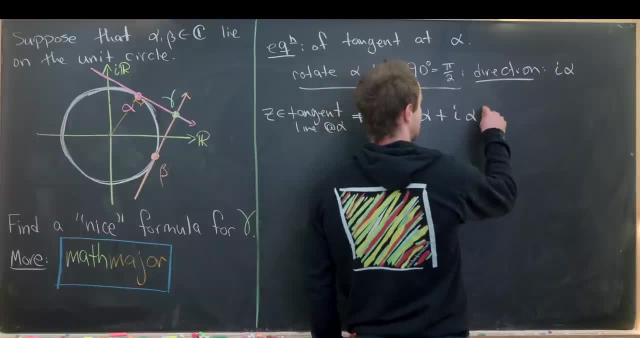 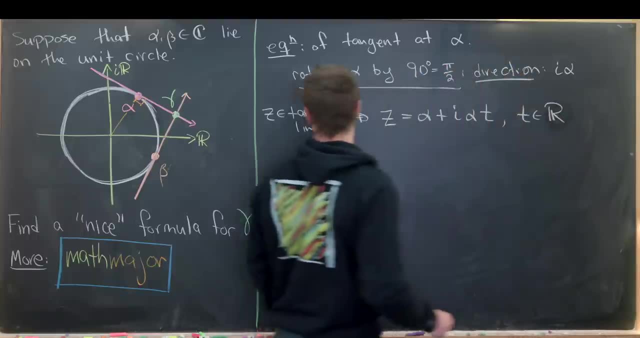 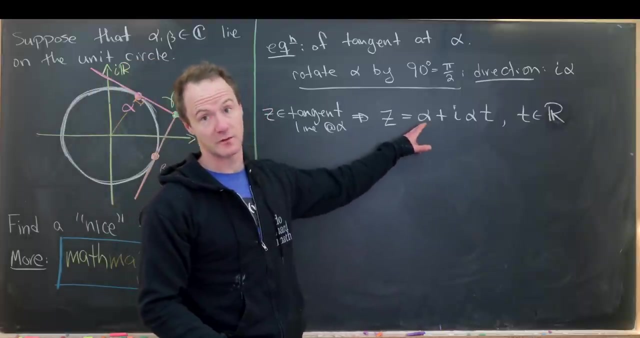 So it's equal to alpha plus i times alpha times t, where t is some real number. So I'll just write: it's some real number. So I think we can talk through that a little bit pretty easily. So notice alpha. the alpha right here just takes us from the origin to this point along. 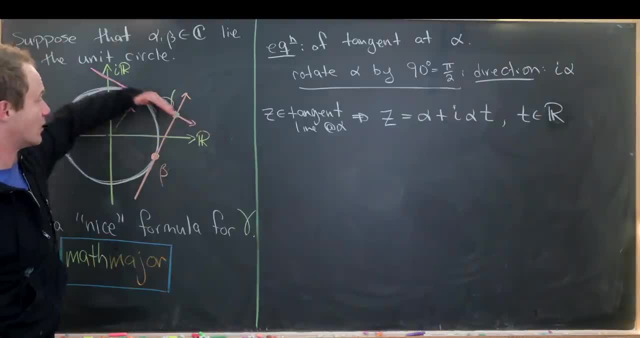 the line And then i alpha tells us that we're going in this direction And then that t tells us how far we're going. So, for instance, if we take t to be maybe negative something just because of how i rotates in this direction, we would get something down here. 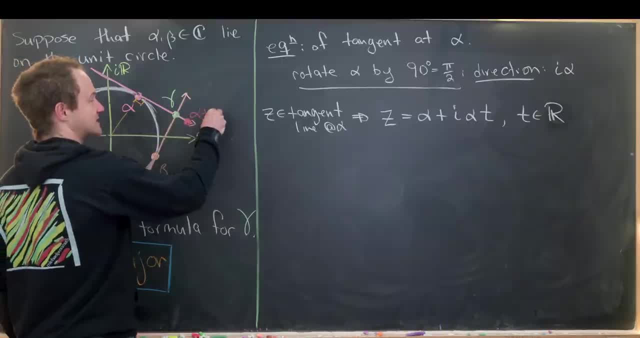 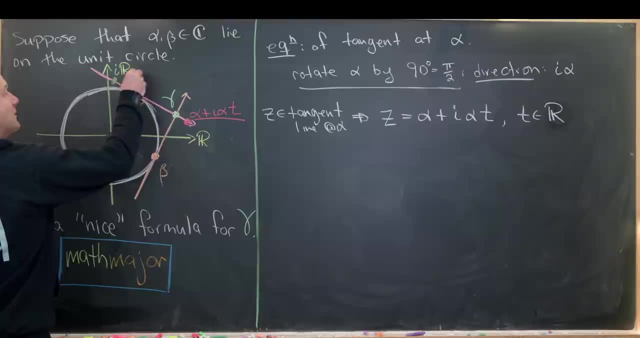 So this would be an example, Okay, Okay, So this would be an example of alpha plus. i times alpha t where t is negative. But then something up here would be an example of alpha plus. i times alpha t when t is positive. 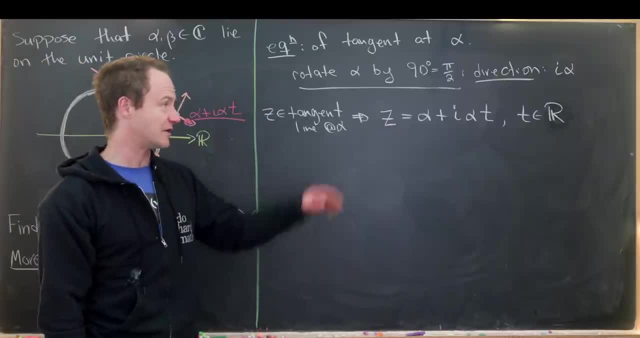 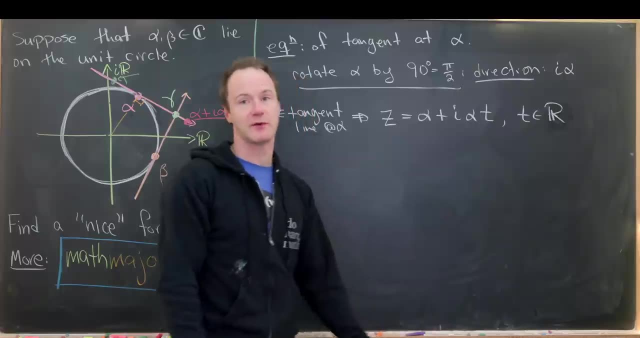 Okay. So anyway, we've got at least a z value for this equation, but maybe we could also remove the parameter, In other words, write this without the parameter t. That would maybe be a little bit nicer. So maybe the first thing we'd like to do is maybe. 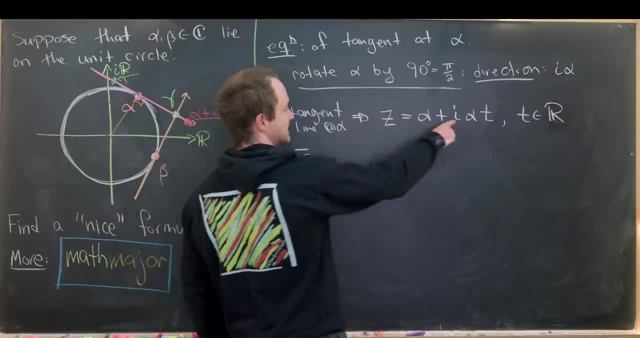 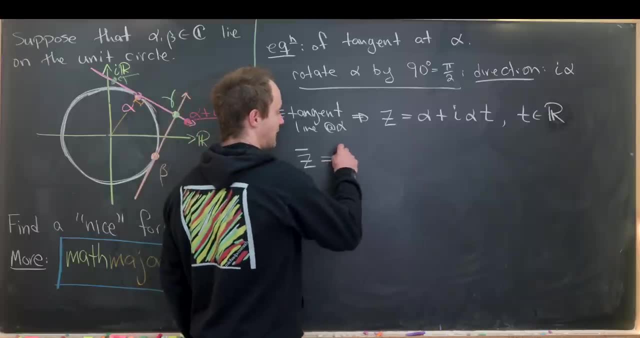 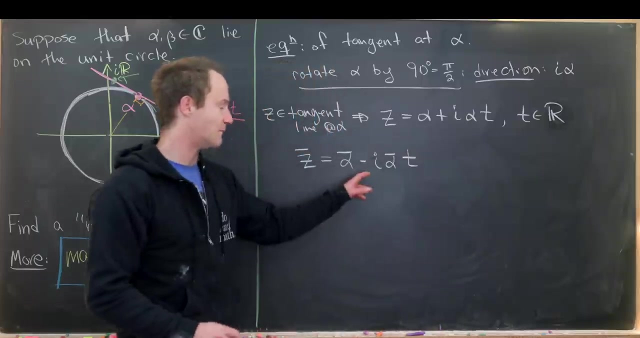 Take the complex conjugate that'll turn this i into a negative i, which looks like it would be along the way to get rid of the t. So z bar will be alpha bar. Recall that alpha is a complex number Minus i times alpha bar, times t. 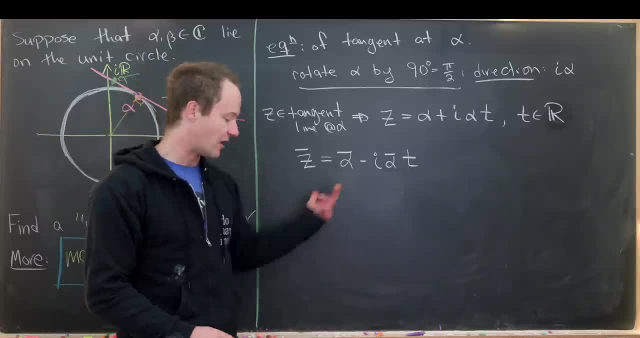 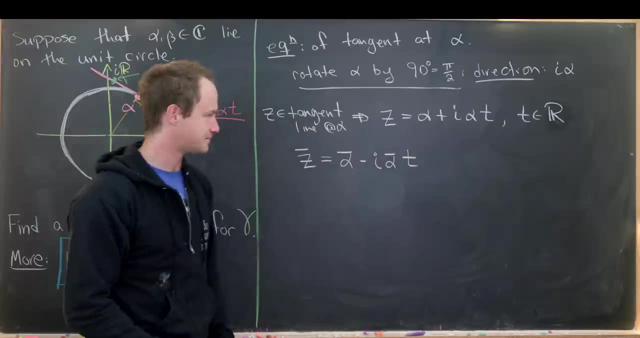 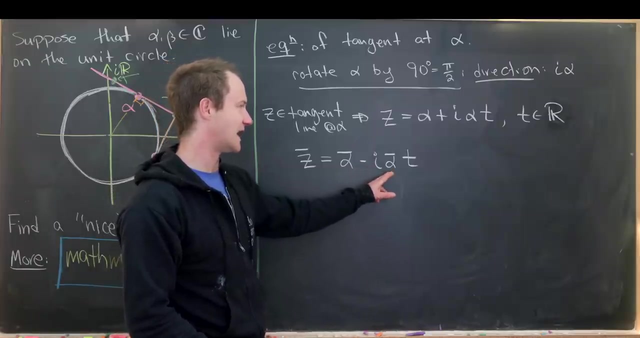 Minus i, because that's the conjugate of i And then alpha bar, because we still need a conjugate of alpha. T is real, So that means that we don't need to conjugate that. So now, looking at this, We see that we have a minus i- alpha bar instead of a minus i- alpha. 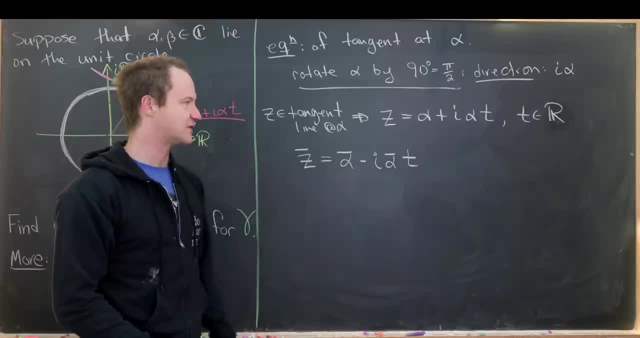 We'd really like a minus i alpha. There's actually a bit of a trick to go from alpha bar to alpha And that will use the fact that the modulus of alpha is one. How do we know the modulus of alpha is one? Because it lies on the unit circle. 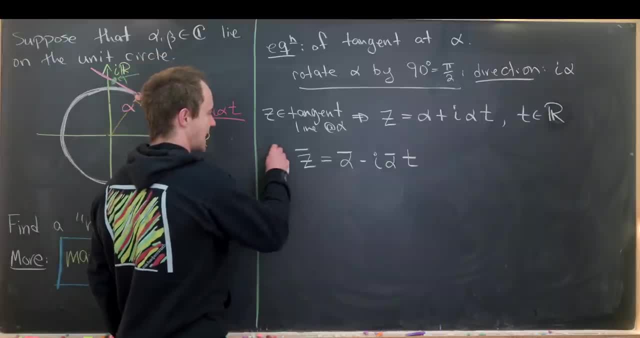 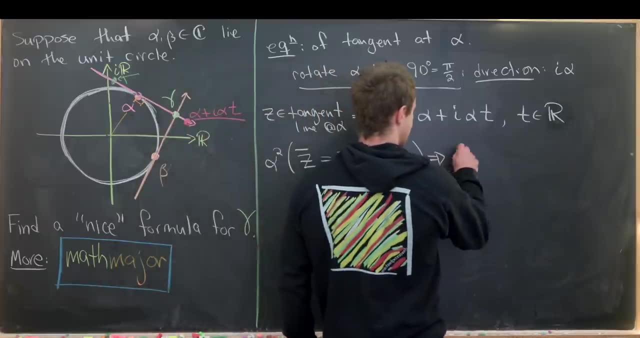 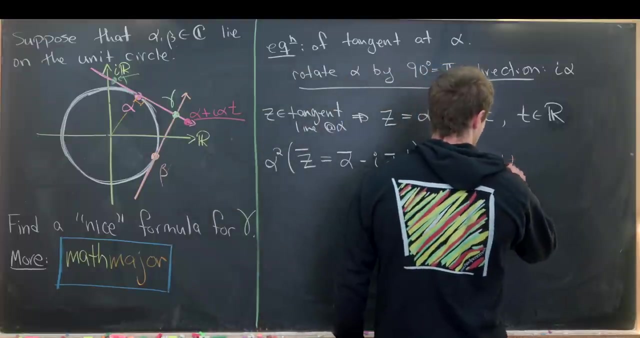 So we hadn't used that yet. So let's multiply this entire equation by alpha squared. We'll see why by alpha squared when we work it out. So this is going to give us alpha squared times: z bar equals. let's see the modulus. 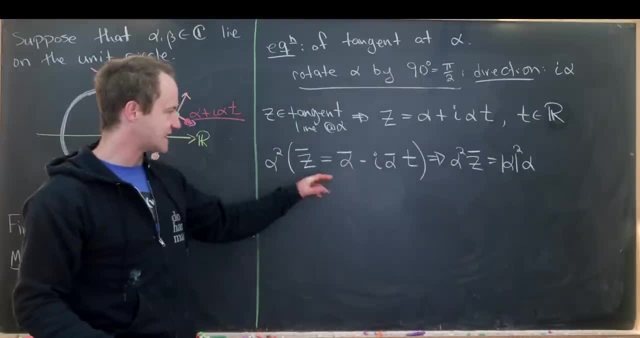 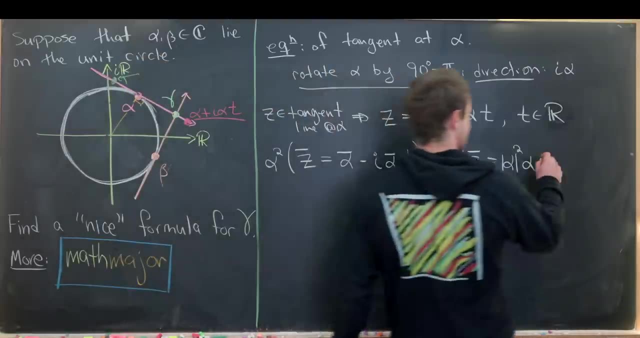 of alpha squared times: alpha. So I take one of these alphas, multiply the alpha bar, That gives me the modulus of alpha squared, And I use the other one just on its own, And then the same thing over here. So this is going to be minus i. modulus of alpha squared times. alpha times t. 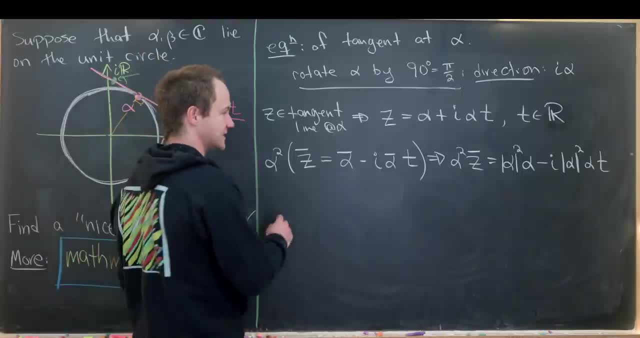 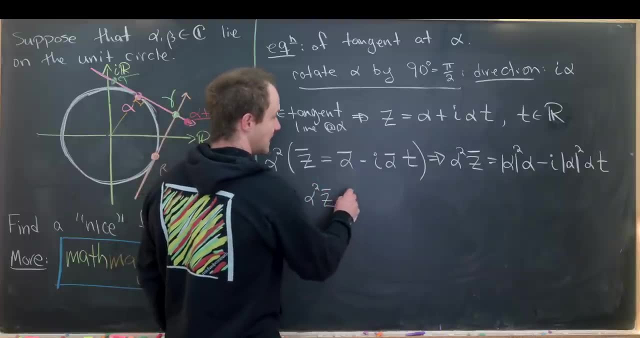 But now, like I said, We're going to use the factor, We're going to use the fact that the modulus of alpha squared equals- what did I say? one. So that gives us alpha squared z bar equals alpha minus i times alpha t. 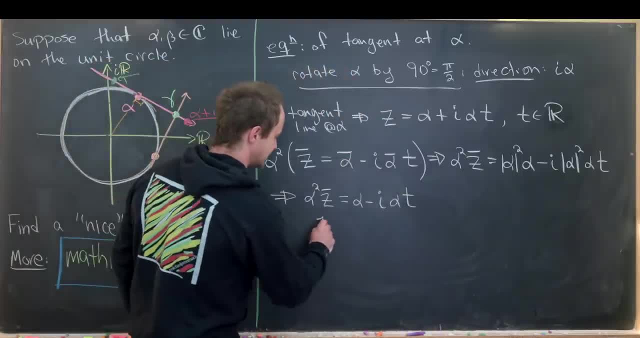 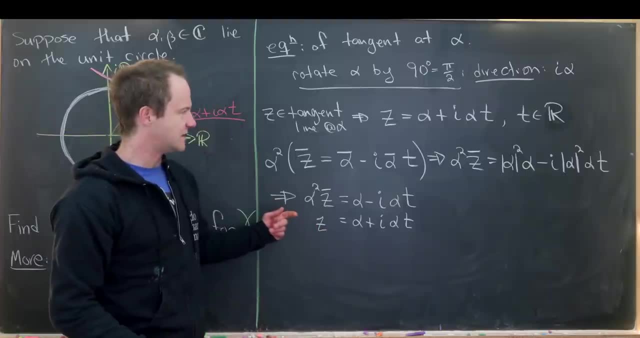 So now let's rewrite this down here, just so that we can see how we'll use it. So we have z equals alpha, plus i alpha t. So that's actually really good news, because what do we have here? Well, we've got something with a plus i alpha t. 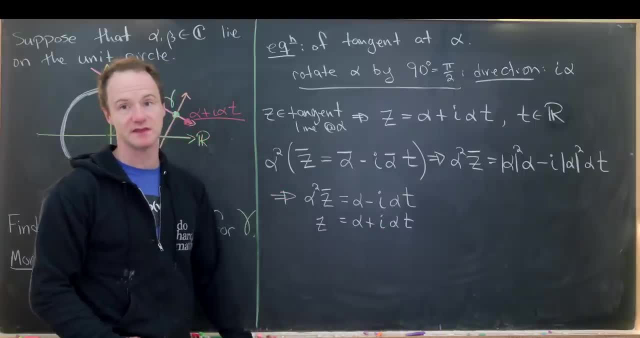 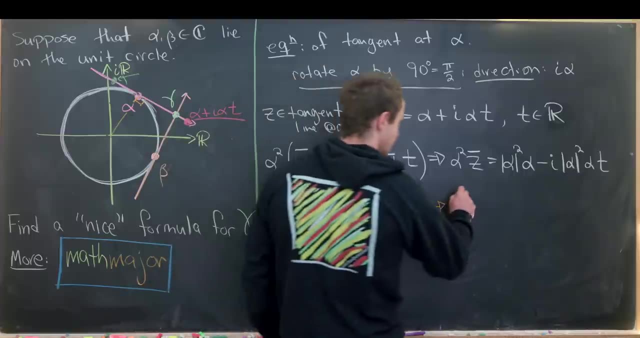 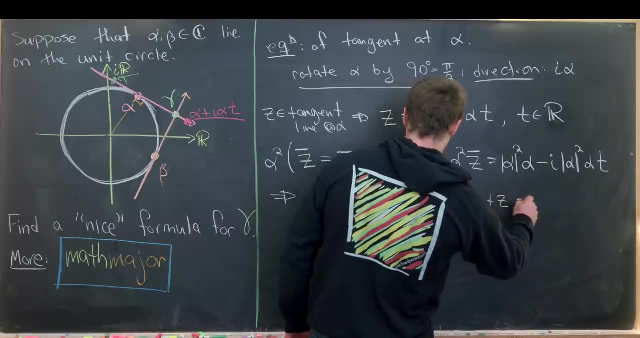 We've got something with a minus i, alpha t, So if we sum these, we will in fact get rid of the parameter, And so let's do that exactly. So if we take the sum of these two equations, we have alpha squared times, z, bar plus z equals. 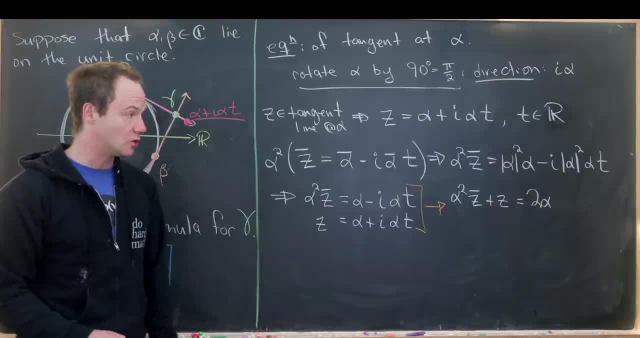 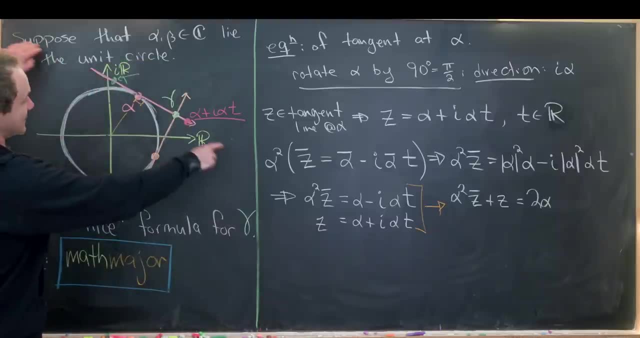 two times alpha, And that's a nice closed formula without a parameter for all of the z values along this tangent line. So we're going to use that to get the tangent to the circle at alpha, which means we can get a similar equation right here for the tangent to the circle at beta, just with beta. 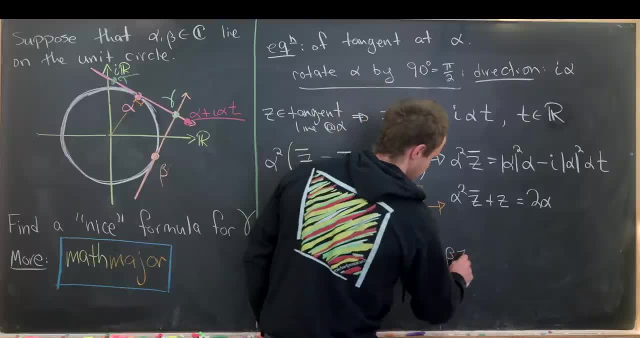 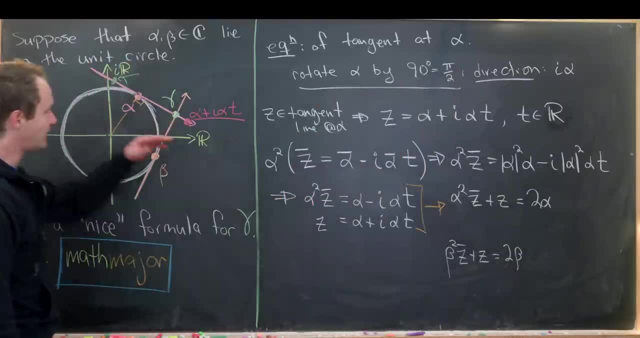 replaced with alpha, or alpha replaced with beta, So the other one will be beta. squared z bar plus z equals two beta. So the alpha one is for this line, The beta one is for this line. So if we're looking for gamma, which is the intersection, that means it must lie on both. 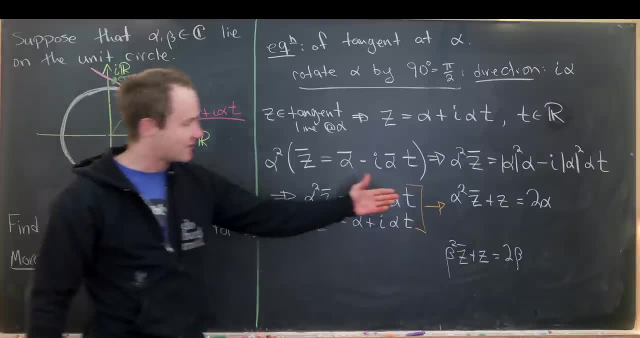 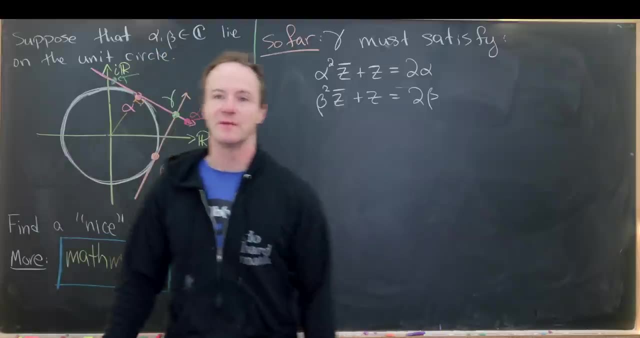 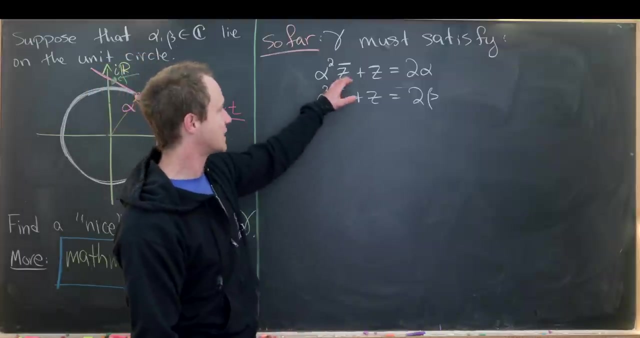 lines. So that means we have to solve this system of equations right here for z, which is exactly what we'll do at the next board. So far, we've determined that this intersection point gamma must satisfy the following system of equations: So we've got alpha squared z, bar plus z equals two alpha and beta squared z, bar plus z equals. 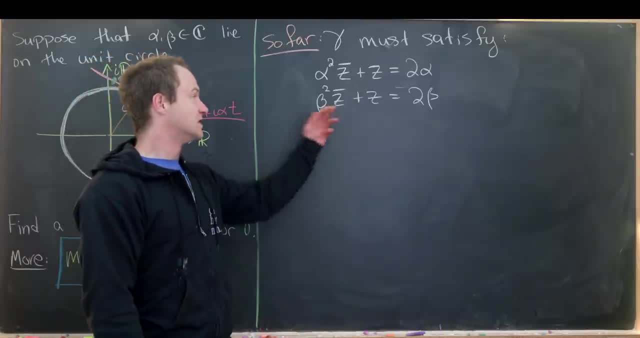 two beta From here. we'd like to maybe solve for either z or z bar. Looks like it's going to be a little bit easier to solve for z or z bar. It's going to be a little bit easier to solve for z or z bar. 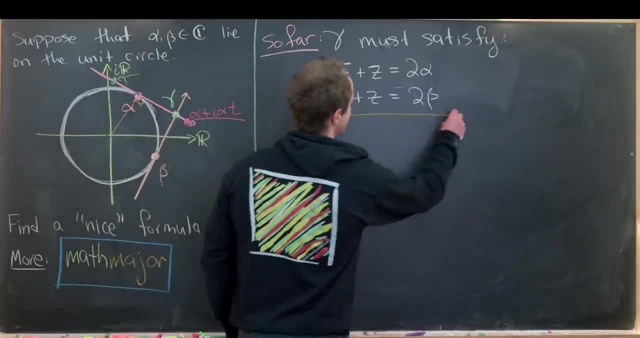 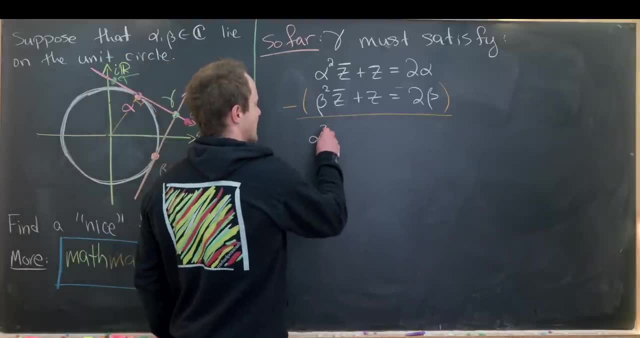 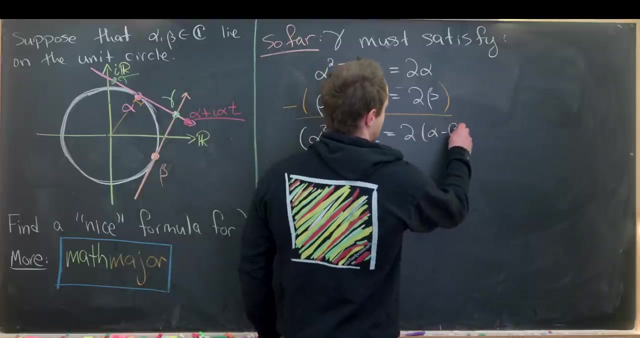 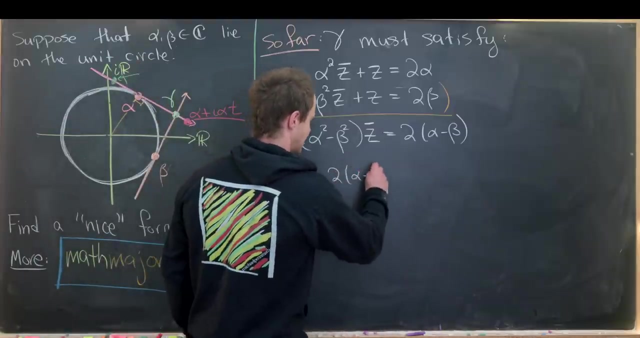 So that's what we'll do. We'll take these two equations and then subtract the second from the first. So let's see, That'll give us alpha squared minus beta. squared times z bar equals two times alpha minus beta. Okay, but that means that z bar is equal to two times alpha minus beta over alpha minus. 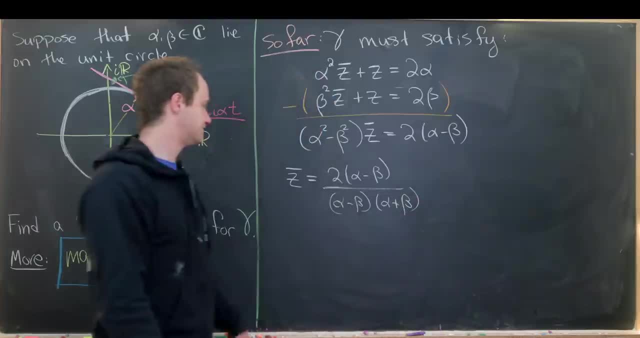 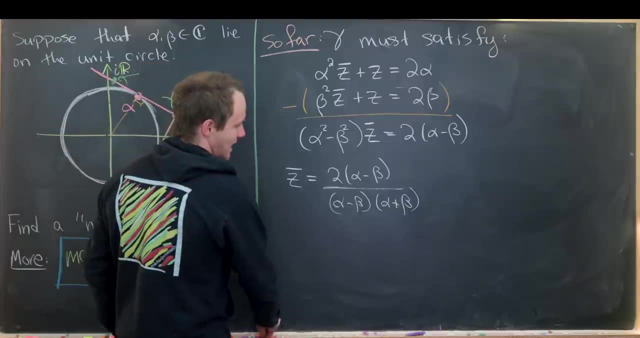 beta times: alpha plus z bar. Okay, So that's going to give us alpha squared minus beta, where here we're factoring this difference of squares using the standard factorization technique. But now we can make a simplification: This alpha minus beta will cancel this alpha minus beta. 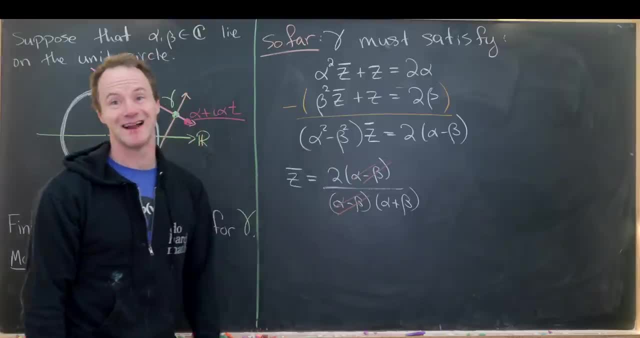 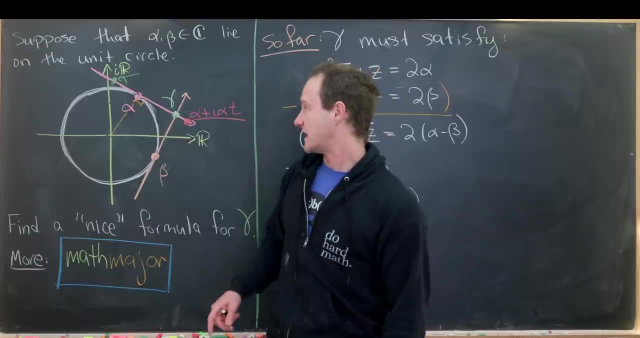 Notice. of course we're only allowed to divide if alpha squared is not equal to beta squared. So that tells us that we can't find the intersection point when, like I said, alpha squared is equal to beta squared. Maybe tell me what that takes out of our ability over here.